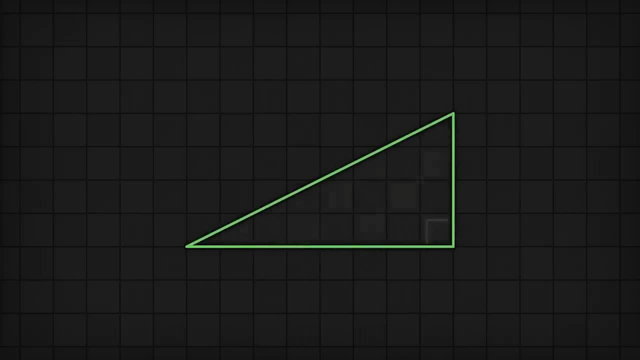 In school I learned the trigonometric functions kind of like this: You have a right angled triangle, an angle typically called theta- here Mathematicians love Greek letters- And you label the sides opposite adjacent hypotenuse. Then you have the famous formulas sine equals. 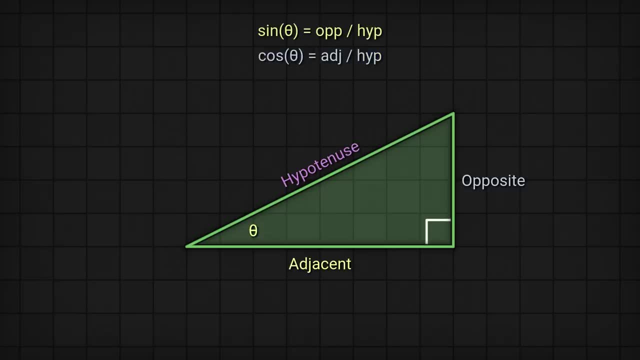 opposite over hypotenuse. cosine equals adjacent over hypotenuse and tan equals opposite over adjacent. So in 20 years of development, even in graphics work, I think for me this triangle has come in handy close to zero times. So instead, another way of visualizing this is: 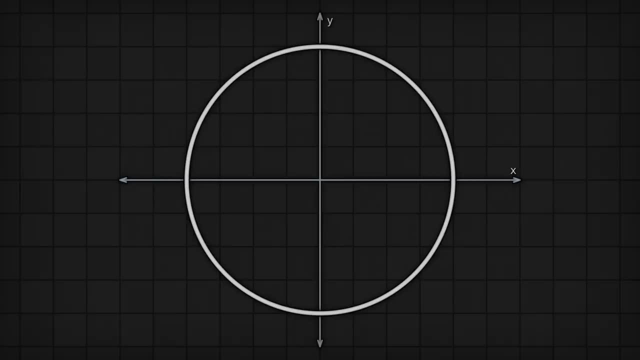 to start with a circle And to simplify things further, we can use one with a radius of exactly one, That is, any point that lies here on the circle is at a distance of exactly one from the center. Typically this angle here between our vector and the x-axis theta. 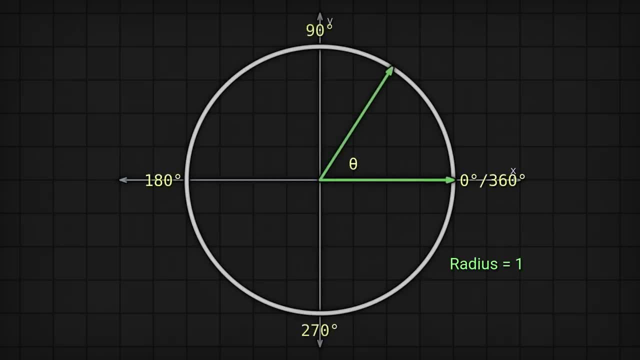 is expressed in degrees ranging from 0 to 360.. But apparently this is some arbitrary system left over from well. they're not quite sure. But if you think about the circumference of a circle that's defined by 2 times pi, times the radius r, With a radius of 1, that 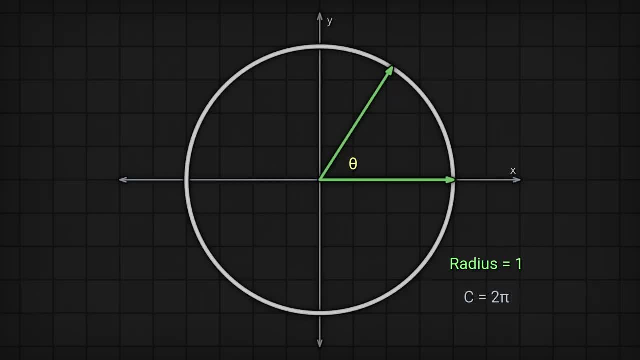 boils down to just 2 times pi. So instead of degrees, if we started at the x-axis here and moved one unit of distance along the circle, we could invent a new unit for angles called a radian. So now we express angles in terms of distance along the outside of the circle, And thus 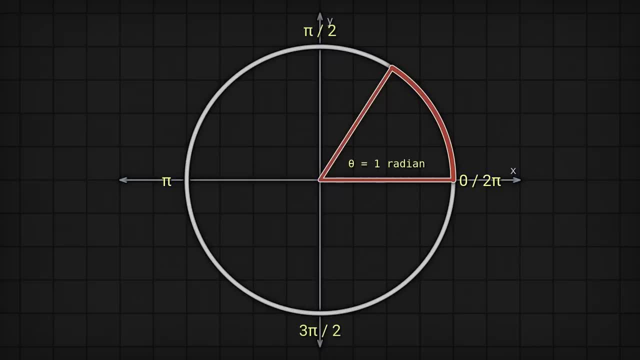 a circle is 2 pi radians instead of 360 degrees, And that's how radians are made. Now, given this point here on the circle, it forms an angle, theta, And since the radius of this circle is 1, the hypotenuse is 1.. So sine is just the distance here along the vertical. 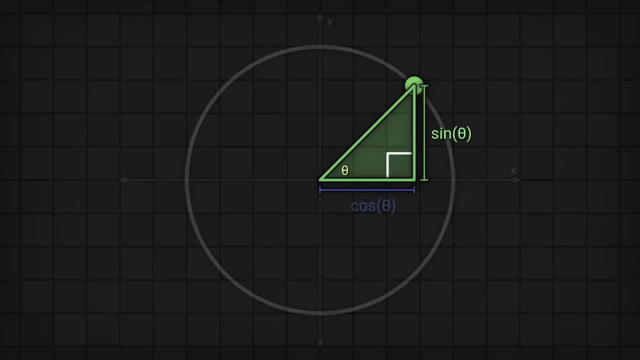 And that means that cosine is just the distance here along the horizontal And tan. Well, you extend a line here from x equals 1 upwards, and you extend the vector forming your hypotenuse out this way: where the two meet, Tan gives you this distance here, The distance from. 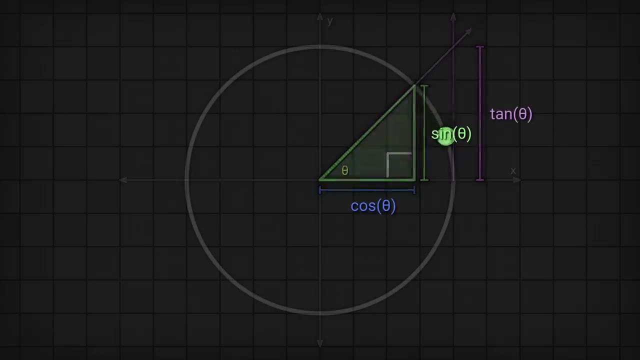 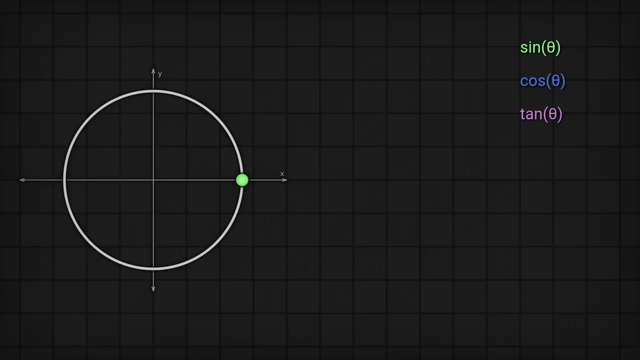 their intersection down to the x-axis. I never used this, but it's there. As you move this point around the circle, we obviously expect cos theta, sine theta and tan theta to change, And we can graph those changes. So sine theta oscillates between 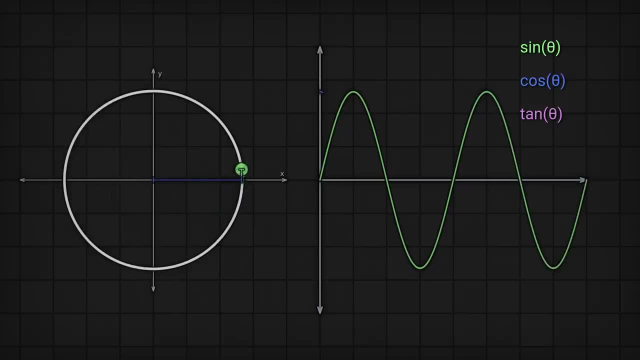 1 and negative 1. Right, oops, I think I forgot that. Let's take a look at the whole thing. 1- as this vector rotates the circle And coast theta oscillates in much the same way but just slightly offset from sine of theta. Tan is interesting because at pi over 2 and negative. 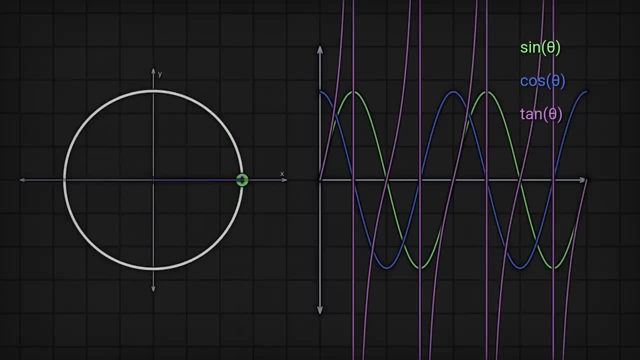 pi over 2, you can see that tan theta is undefined. Hopefully now, seeing this in action and what tan really is, the graph of tan theta makes much more sense Why it kind of freaks out at certain values. This is where it gets a little interesting If we call this vector. 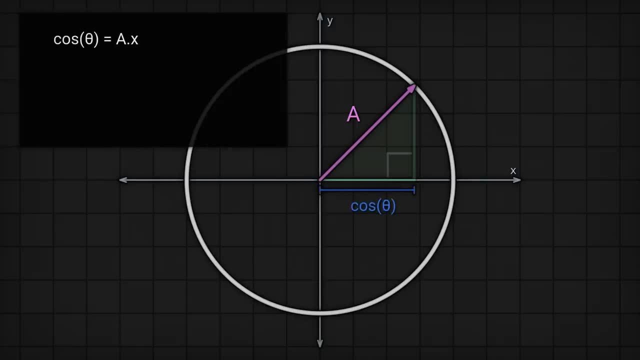 a. we know that coast theta is just the x component of this vector here on the unit circle. Or you could say this in a different way. A slightly longer way of saying it is in terms of the full vector a: It is a dot x times 1 plus a dot y times 0. Or again: 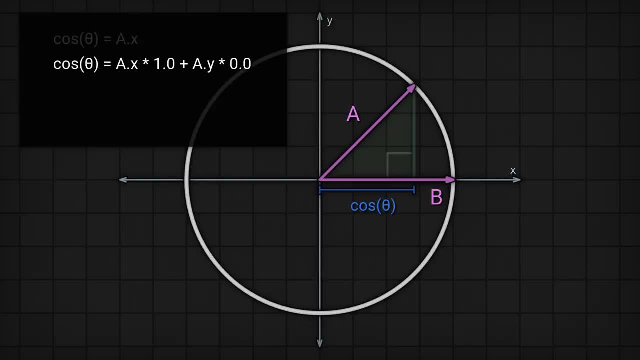 now we can say it in terms of both a and b, where you know the b vector is just the x axis or 1: 0. So it's a dot x times b dot x, plus a dot y times b dot y, Which is now defined in a more mathematical way. It has a name, It's the dot product. 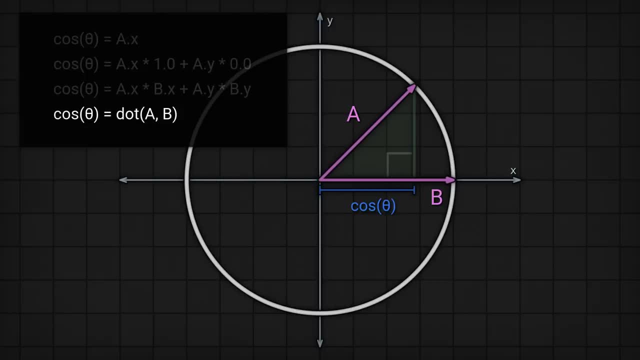 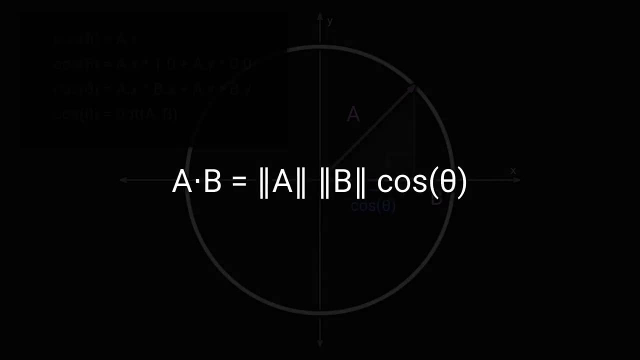 So the dot product of a and b is equal to coast theta, Which is just this horizontal distance here if a and b are unit vectors. The more general equation you were taught in school was that a dot b is equal to the length of a times the length of b times the. 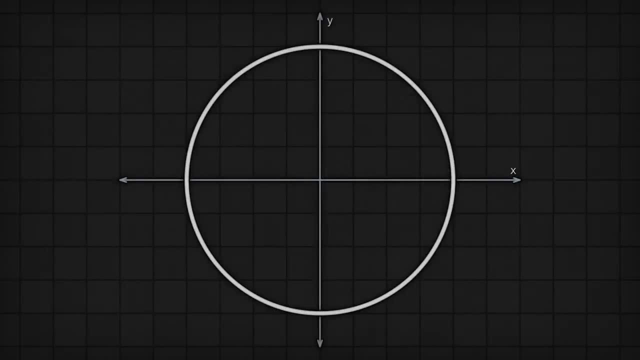 coast theta. So now it might make more intuitive sense for why, given any two unit vectors, if we take the dot product between them, we then have one product of a and b, that's the dot product of b times the length of b times the coast theta, Which makes much more sense. 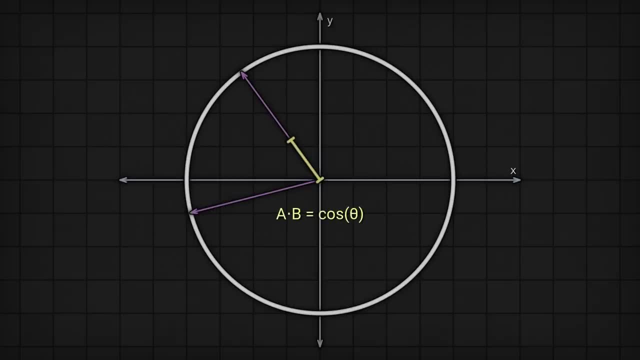 for what we need, you get cos theta, Because if you were to rotate these things around the circle until one hits the x-axis and suddenly this is just reduced to our simple distance along the x-axis, Actual, real proofs exist with like real math and everything. This isn't one of them. 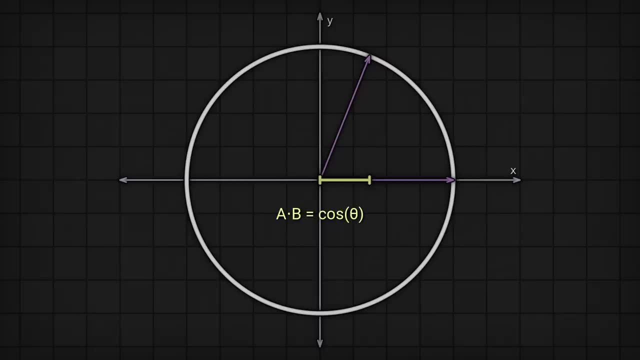 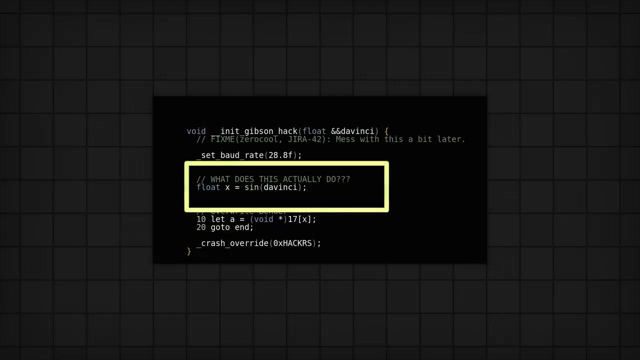 just a nice way of visualizing things, But this is also why the dot product is used to get the scalar projection of one vector onto another, because that's all this distance is. So then, how are these functions implemented If you have a chunk of code when you call your hardware or 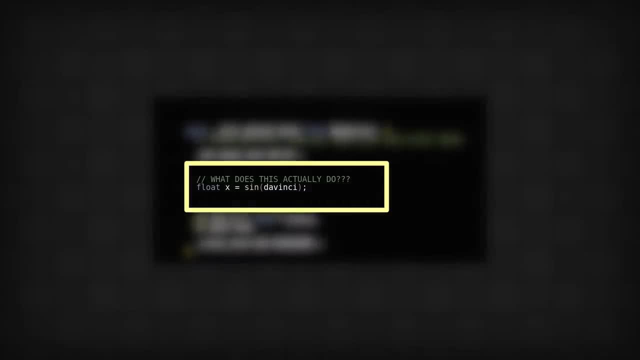 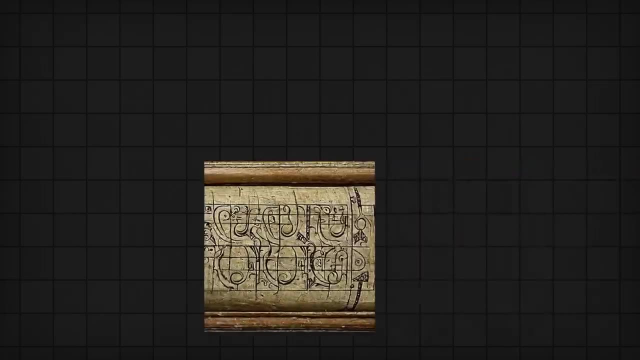 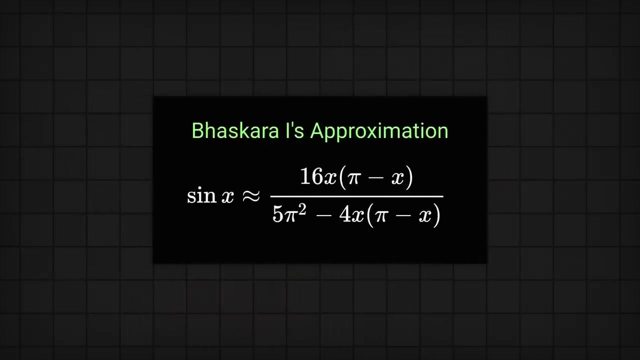 library function for stuff like sign. what kind of math sorcery are they doing? Well, these tend to be computed in different ways. Various approximations have existed for ages. Back in the 7th century, the Indian mathematician Bhaskara gave the following formula, which I'm 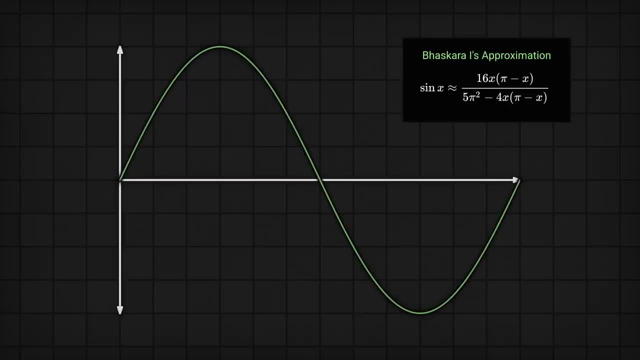 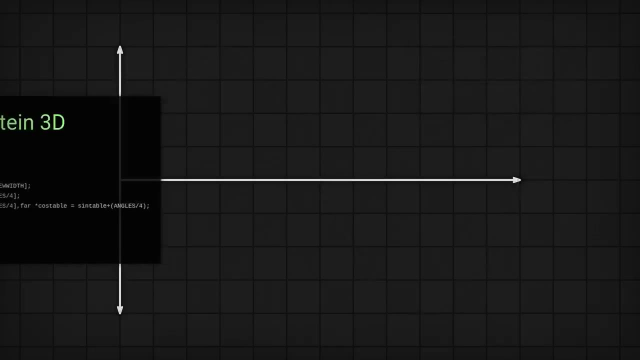 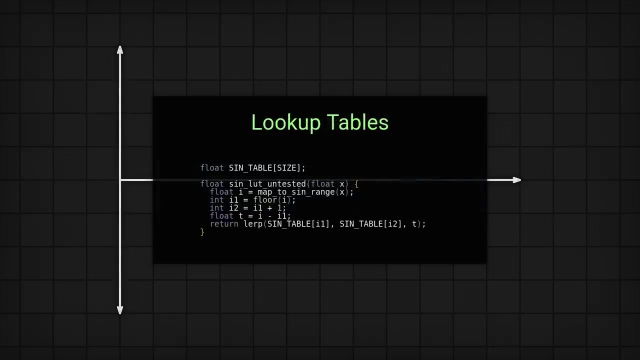 not going to read, but it worked really well in the range of 0 to pi, giving an absolute error of 0.0016.. In game development way back in the day, it was often acceptable to use something called a lookup table By pre-computing values and either finding the closest match or linearly interpolating. 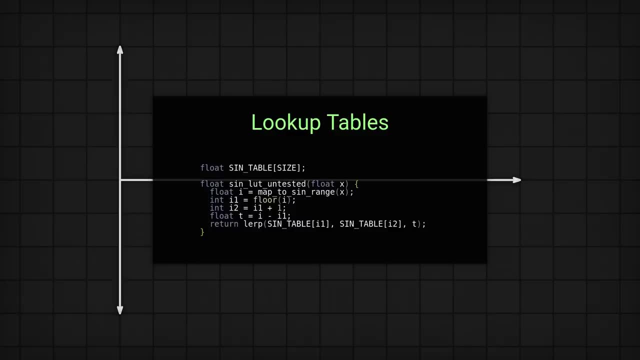 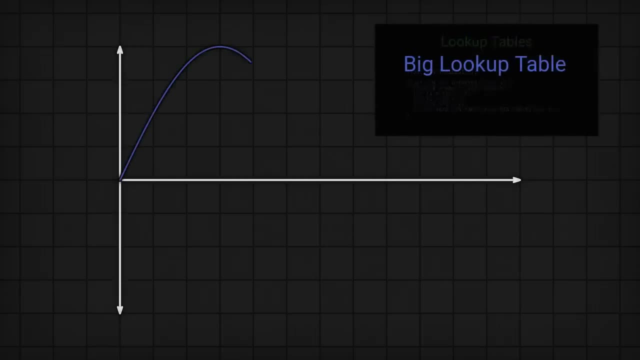 between adjacent values. it was possible to use a relatively small lookup table to get acceptable results. A lookup table with 512 entries might have an error of around 0.00001, or 1e to the negative 7.0.. If you have a lookup table with 512 entries, you might have an error of around 0.00001,. 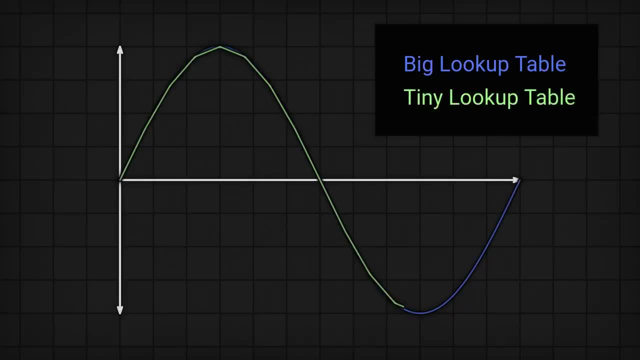 or 1e to the negative 7.0.. But getting things super right in games isn't usually critical. No one's life is on the line unless you're Jigsaw. So, for example, you could use 16 values from 0 to pi over 2, and that gives an error of 0.0014.. But cache misses are expensive these days. 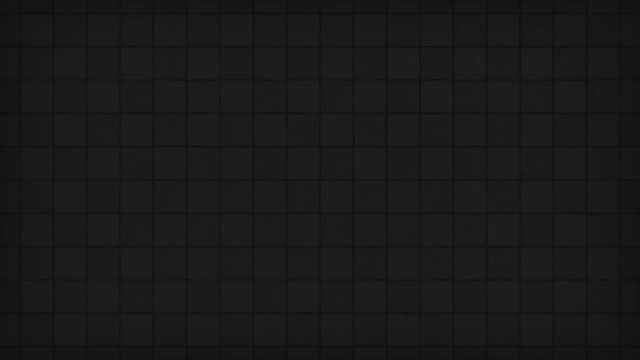 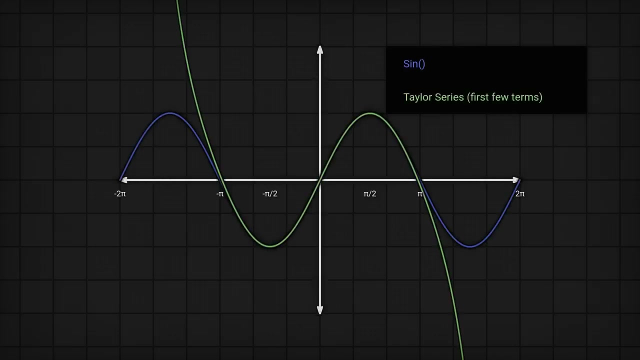 so lookup tables aren't used as often anymore. If you were to compute these trig functions directly, the first thought is a Taylor expansion, and courtesy of Wikipedia they look like this, which does the job. But a common complaint with Taylor series is that the error isn't uniform. The error scales the. 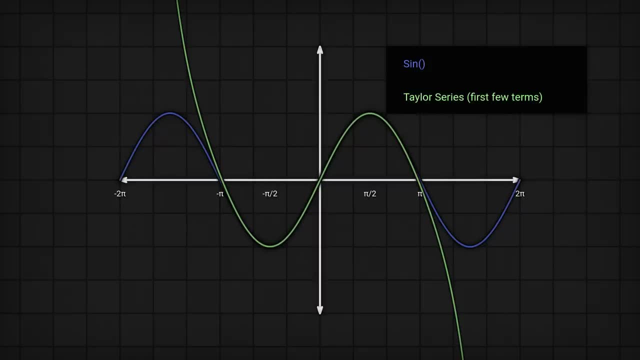 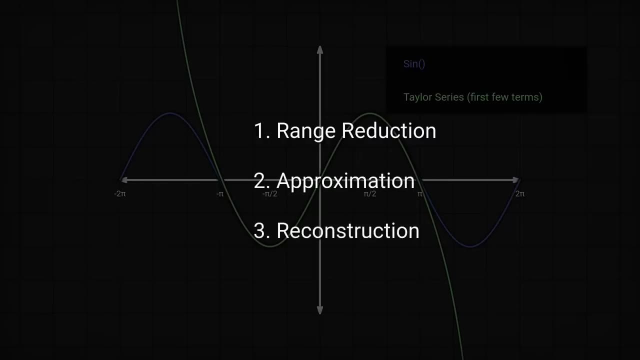 further, you are from 0.. Better approaches have a general theme. They combine a whole bunch of ideas. They tend to do what's called a range reduction followed by an approximation and then a reconstruction step. First off, looking at a sine wave, you clearly don't need to approximate. 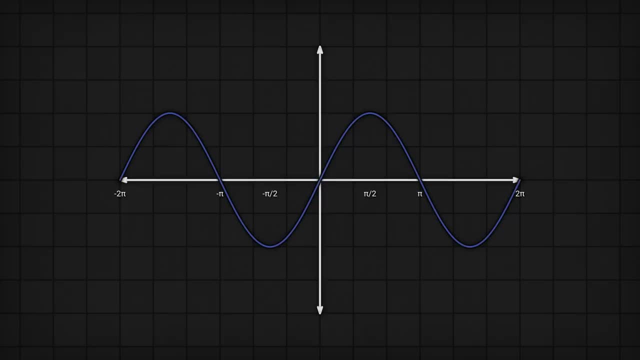 from negative infinity to infinity. We already know that it repeats after 0 to 2 pi. From there you can exploit symmetry. This half is really the same as this half, just upside down, And this half of the wave is really just a mirror of the other side. So in reality you only need to approximate.